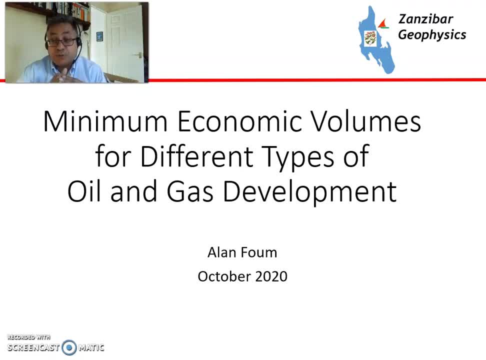 Hello, my name is Alan Foom and today I'm going to talk about minimum economic volumes for different types of oil and gas development. The key point of this presentation is to enable a geologist to be able to talk effectively with engineers, with economists, so that you can talk. 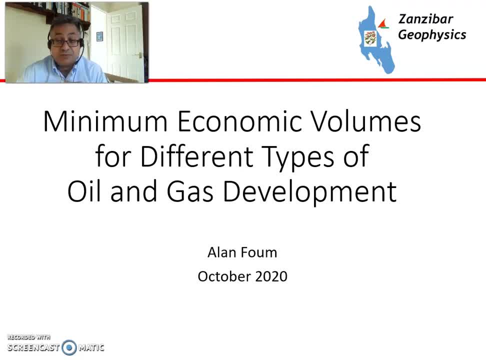 about what sort of volumes can work for your prospects. So, for example, if you have a very small prospect in a remote area which is unlikely to work because it's just too small, you'd know about it before going to an engineer and saying can you have a look at this? So these are indicative. 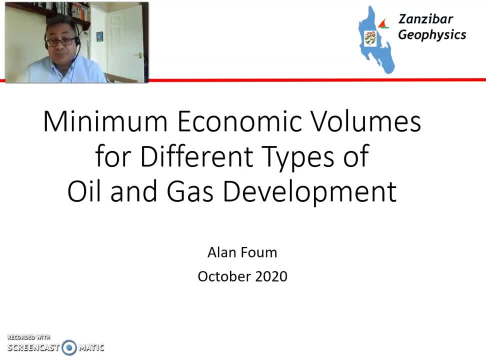 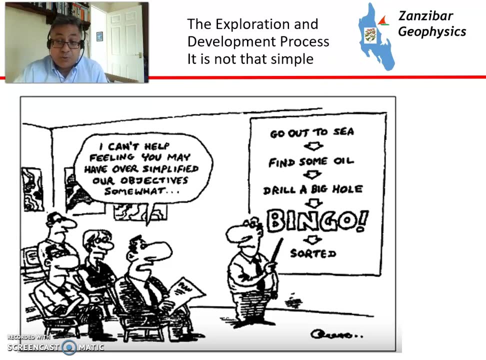 numbers and I would strongly recommend that you talk to professional engineers and professional economists during your prospect definition. but this is indicative numbers to enable you to have an effective conversation. Now, this is what most people think exploration development is like, but we all know it's not as simple as that. You don't just go out to see find some oil drill. big hole bingo sorted. There are an awful lot of things that you can do to help you get the most out of your prospect. You don't just go out to see find some oil drill. big hole bingo sorted. There are an awful lot of. 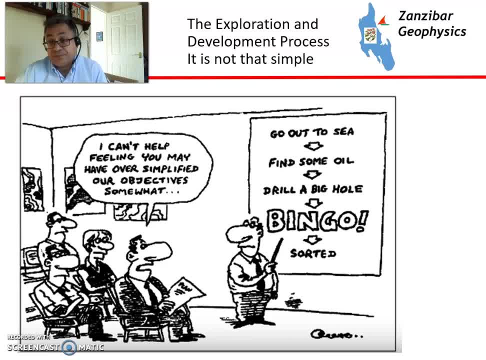 highly skilled professional people who all work together to make these things happen. And in order for you to be able to work effectively, you need to have an understanding of what other people are talking about. Obviously, you won't be able to do their jobs anywhere near as good as them, but you will understand what they're saying, so you 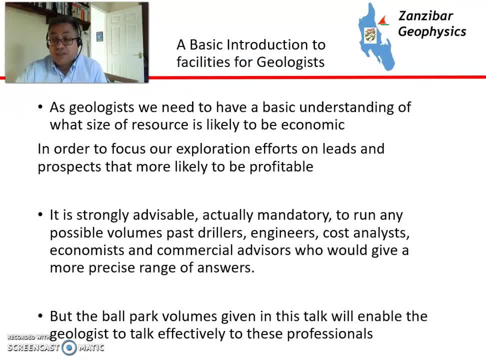 can have effective conversations. So strongly advisable to talk to the engineers, but these ballpark volumes gives you an idea of what could work where. So this is gleaned from Perth, my 20th year of professional experience working for an oil and gas major. 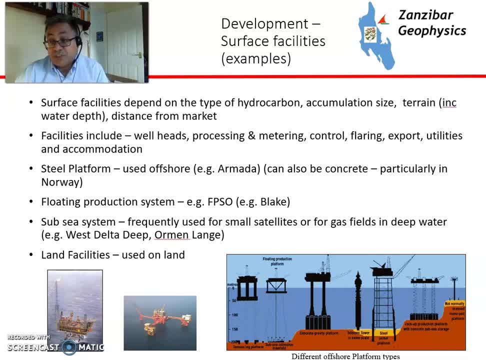 So facilities are dependent on many things. So first of all, this hydrocarbon type, whether it's dry gas, wet gas, condensate, black oil, volatile oil, et cetera. Accumulation size, the terrain including water depth, distance from market et cetera, All of these things. 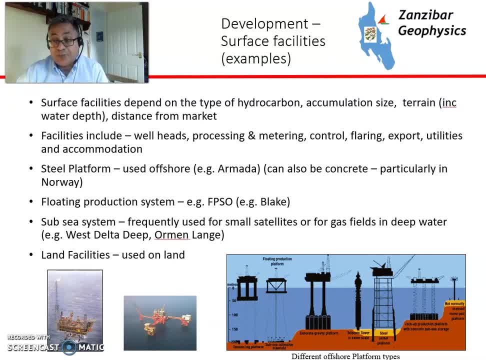 go into there. Facilities that you will need will include wells, wellheads, processing and metering, control, flaring, export- all the utilities and accommodation that people will monitor this day to day. Offshore people can tend to use steel platforms, So this is a picture. 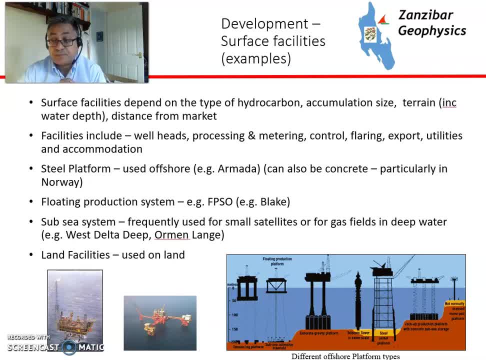 of the Armada platform, which is one of the projects I worked on, But it can also be concrete. Norwegians, in particular, are keen on concrete Also: floating production systems, subsea systems and, obviously, land facilities when you're working on land, And here's a picture of how big these. 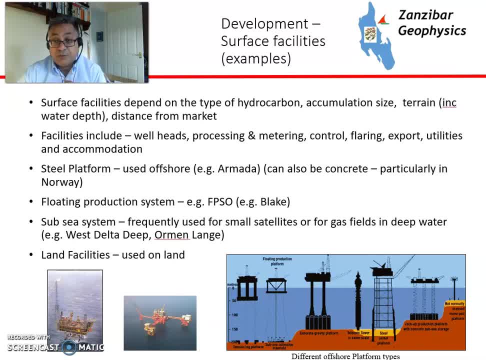 facilities are. I remember going to Newcastle to see the Judy platform being built in 1994.. It was a bright, sunny day in the autumn and the shadow reached across the tide to Jarrow. These things are massive. They also cost a lot of money, but they make a lot of money for you. 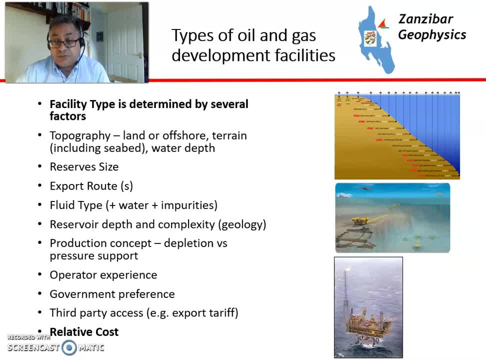 So you're looking at the topography: reserve size, fluid type, reservoir depth and complexity, which is where you come in as a geologist, the production concept, whether you're going to be using depletion or pressure support. gain from your engineers your experience as an operator. 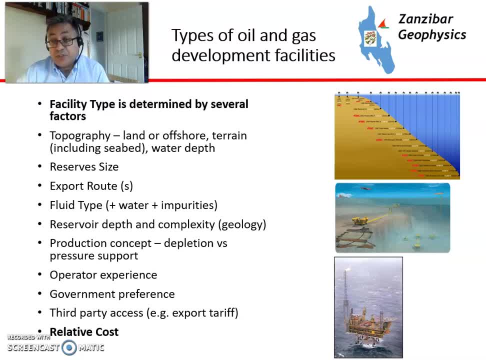 If you're, as an operator, are due a particular type of technology, well, you're likely to use that ahead of other technologies. So, for example, if you're good at subsea, less good at platforms, you will tend to go the subsea. 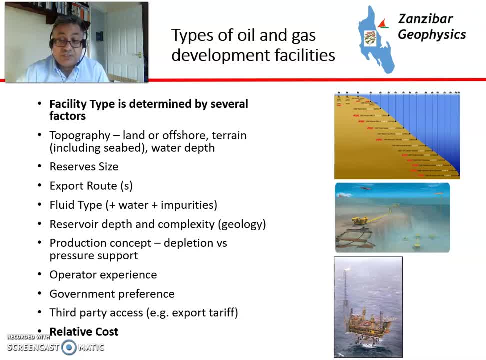 route. more often than not There's also government preference. For instance, the US Gulf of Mexico doesn't tend to be looking less favorably on FPSOs, So the local laws et cetera to be taken into account, And then the influence of third parties. What's growing in the UK at? 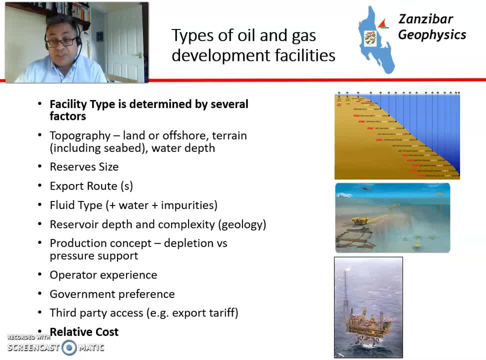 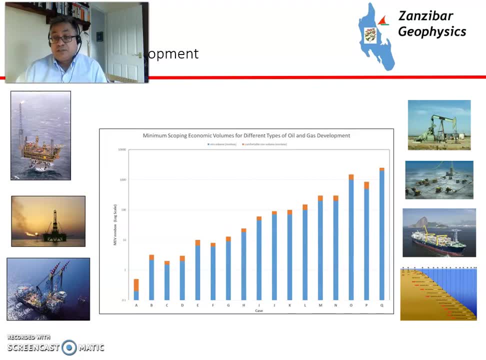 the moment is a desire to have availability for third parties to tie in satellites developments so that infrastructure is used more effectively. So this is something I put on LinkedIn: looking at different charts. So this is a case of looking at different cases, So I'll take you through each one of them in a little bit of detail to show you. 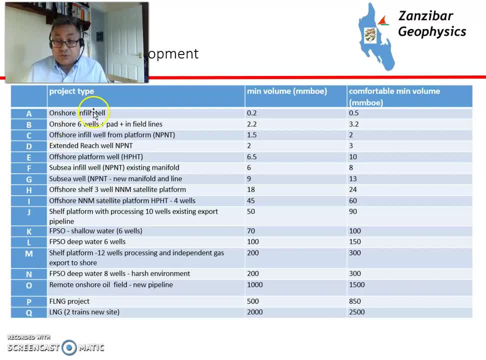 where we are. So look at onshore infill wells- single well, Offshore wells, onshore wells within a pad, Offshore infill wells, extended reach wells, subsea wells not normally manned, subsurfaceroffen, deep water platforms, shelf platforms, FPSOs- deep water FPSOs- remote fields. 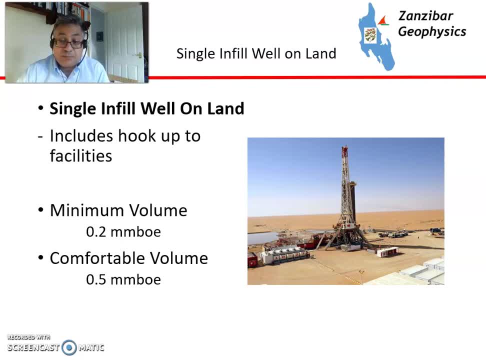 and LNG. So at the lowest level, between 0.2 of a million barrel of oil equivalent or to 0.5 of a million barrel of oil equivalent expected ultimate recovery, you will have a single infill well in line. So this is typical of what you would get for a shale oil well or shale gas well. 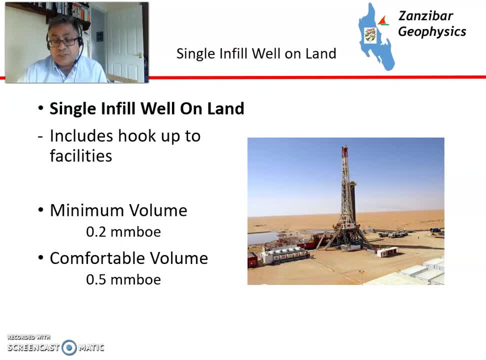 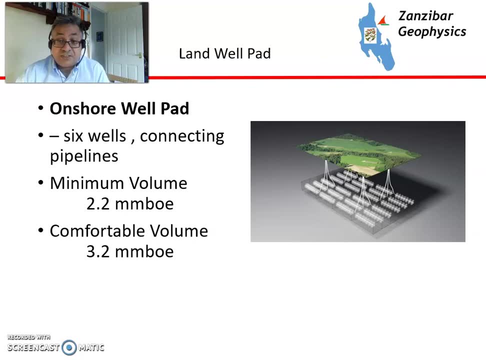 in America people can make volumes that are slightly lower than that work, but this is roughly the amount that you'd want to have to be comfortable. Our land well pad is a situation. we have several wells and here's a picture of land well pad from a. 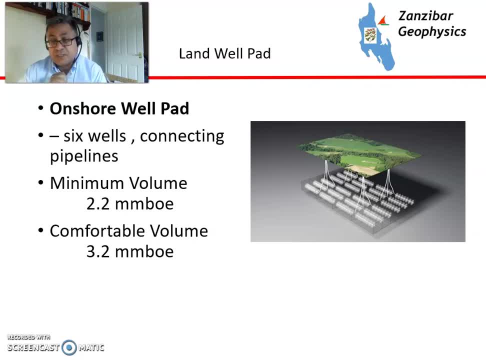 single area. The pad is normally the size of a football field. The well would have some connecting pipelines, the well heads an area for various operations etc. and the minimum volume for a pad would be about 2.2 million barrels of oil equivalent. You'd really want about 3.2 million barrels of oil equivalent to be 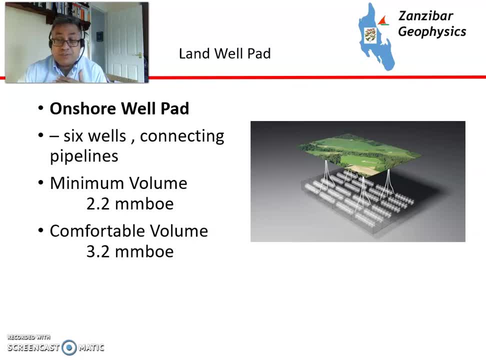 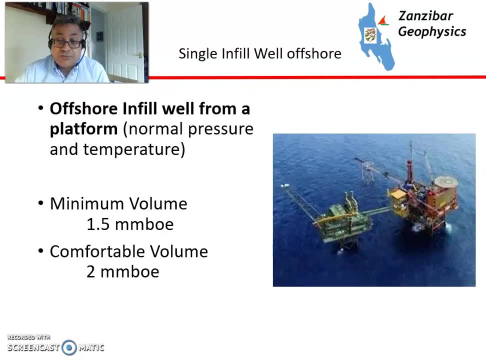 comfortable for all the infill well work etc. Obviously, on top of that you can add wells later at a slightly lower rate, Going to an offshore infill well. so this is from a normal pressure, normal temperature. you'd want about one and a. 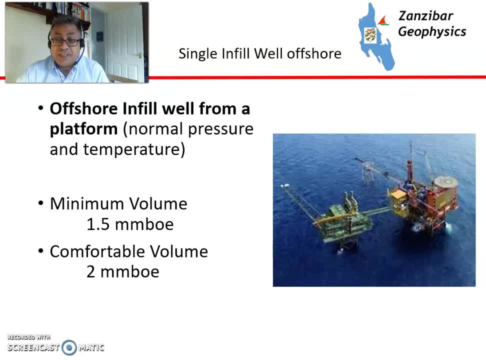 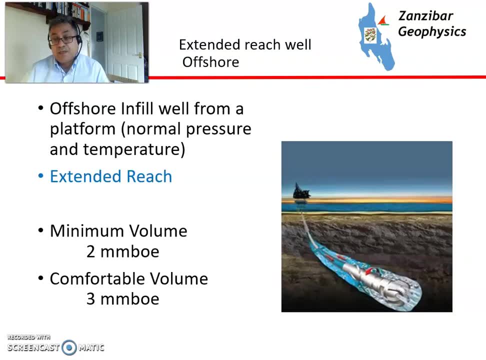 half million to two million barrels of oil equivalent, typical for the North Sea, maybe a little bit less for others. Again, drilled from an existing facility keeps your production profile up. An extended reach well, obviously takes longer in terms of drilling time. so your capex will. 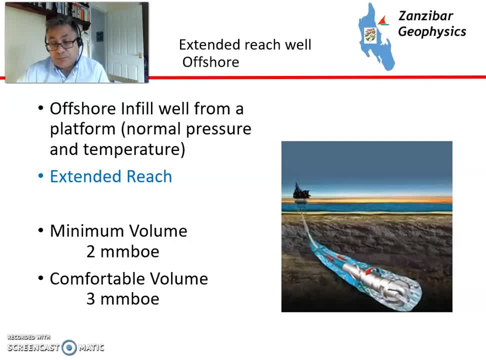 be slightly larger, so your minimum volumes will be between about 2 million barrels of oil equivalent. You'd want about 3 million barrels to be really comfortable. Again, depends on the scale of the well, the complexity of the well, etc. but this gives you a rough idea of where things are Moving to high. 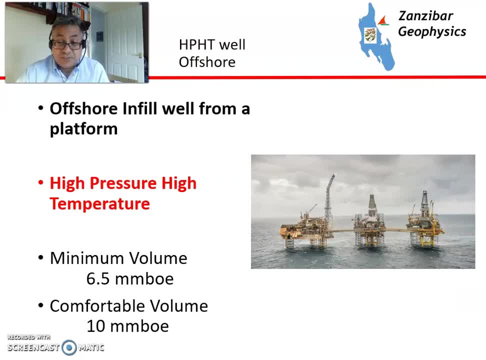 pressure, high temperature, where everything is much more expensive because of safety concerns. so there's a picture of Elgin and Franklin again, another project I've worked on. Now here's what I can say about it. A minimum volumes for an infill. well on a. 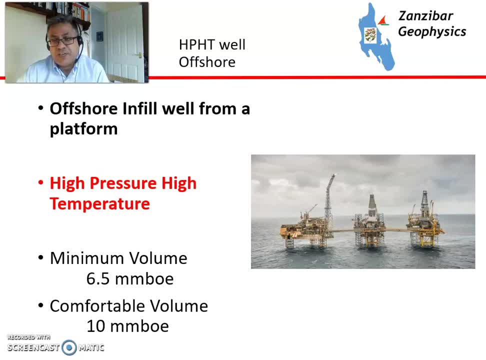 high pressure, high temperature area would be about six and a half, seven million bars of all, equivalent that you'd really want, about 10 million barrels of oil equivalent to to give you a bit of safety margin. Again, complicated wells take a long time, with a lot of complexity and more costs. 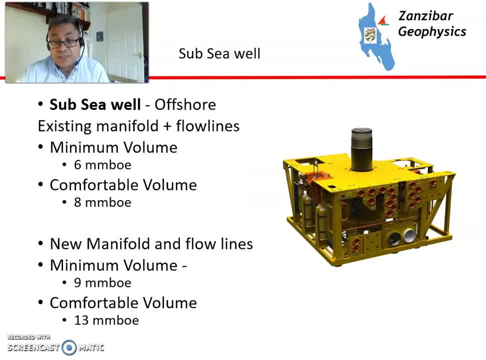 Subsea wells. now subsea has opened up significant portions of the deep water. for example, you've got a manifold and flow lines etc that you'll plug in. For an existing well you'd want about 6 million barrels of oil equivalent to justify it, but for a comfortable volume you'd 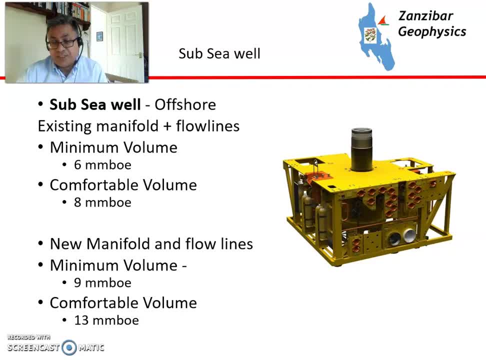 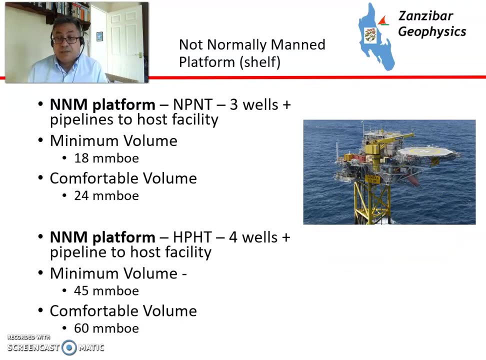 want more like 8. With a new manifold and new flow lines you go to 9 and 13.. Again, depends to some extent on the drilling depth and its fluid types etc. but these are rough ballpark figures to enable you to see if something is likely to be able to work. Looking for not normally. 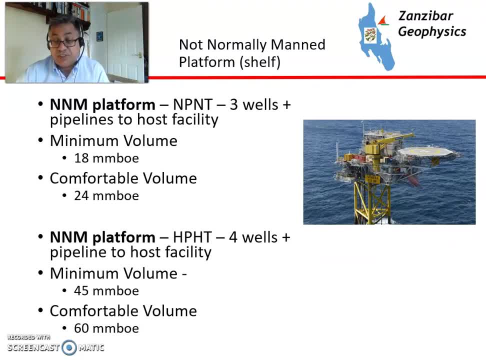 planned manned platforms. so this is a situation where you have a platform that does not have people on it normally, although obviously it could be accessed, as witnessed by this picture, with a helipad. Minimum volume for normal pressure, normal temperature, three wells- you'd want about 18. 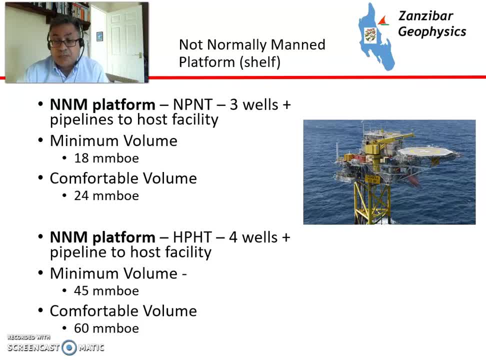 million barrels of oil, equivalent to 24 million, to be appropriately comfortable With high pressure, high temperature, where you have significantly more costs, both in terms of engineering and in terms of the wells, against higher safety risks, with a pipeline to a host facility. you'd want about 45 to 60 million barrels of oil equivalent to be to be really safe. 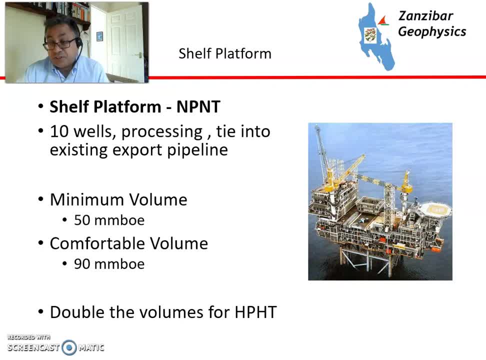 Moving to a shelf platform, normally pressure, normally temperature. so this is a picture of the Judy platform, again another project that I've worked on. So let's say the shelf platform has 10 wells with processing tied to existing pipeline. you'd want a minimum of about 50 comfortable 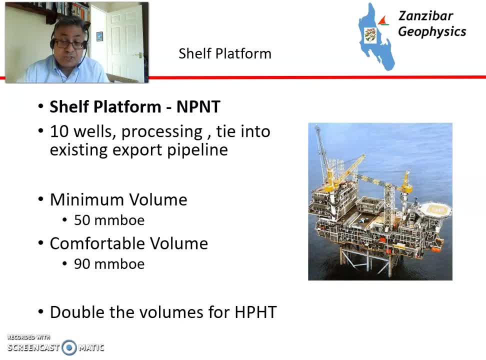 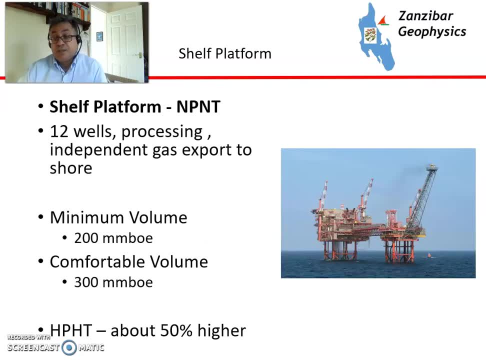 volume would be 90 to 100 and if you're looking at high pressure, high temperature, you want to double those Depends also on the country and fiscal regimes, etc. If you got a shelf platform that has a gas export pipeline. this is another project that I've worked on: Everest in the North Sea, which is the 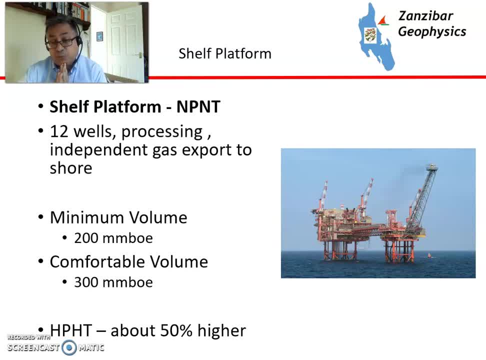 central hub for the CATS pipeline. you'd want about 200 million barrels of oil equivalent, 300 million barrels of oil equivalent to be really comfortable. So that's, you know, slightly over, slightly over tcf of gas. 1.2 tcf of gas to one and a half tcf of gas. It's be higher for high pressure high. 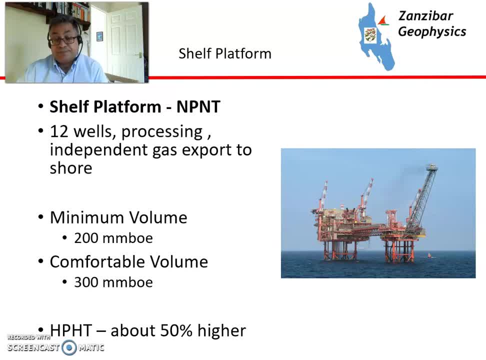 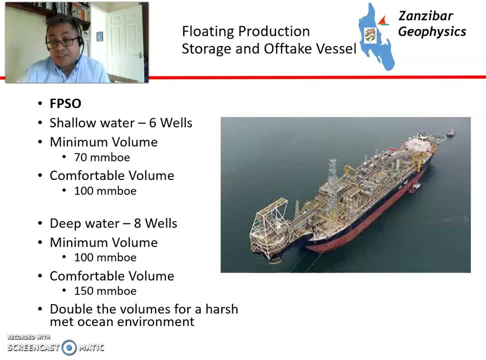 temperature, obviously, because all the costs become become greater. If you're looking at FBSOs, this is very much dependent again on the type of FBSO you have, whether it's a leased FBSO or whether it's a bespoke FBSO which you own. Shallow water with about six wells you'd 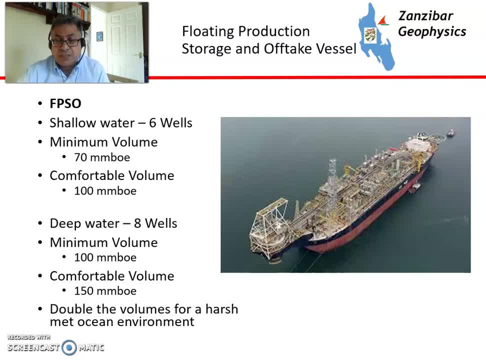 want 70 to 100 million barrels to be fully comfortable. Deep water costs go up a bit, so you want about 100 to 150.. If you've got a harsh ocean environment, you'd probably want to double the volumes for that, Again dependent to some extent on the type of FBSO and the deal that 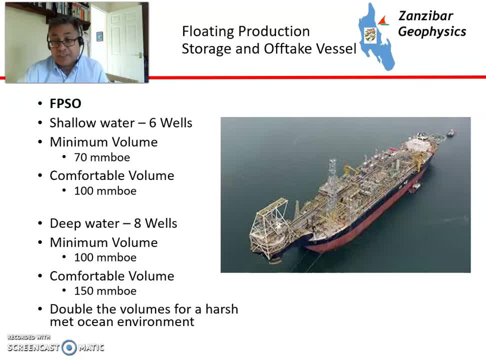 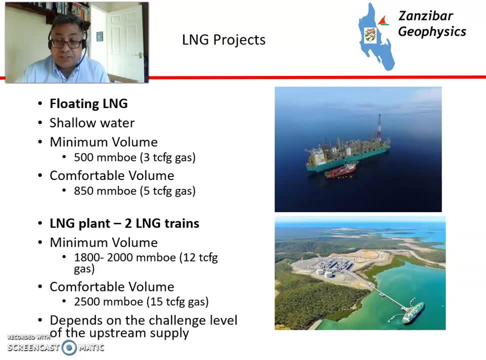 you can make and in terms of acquiring it, whether it's a wet lease, a dry lease or a bespoke ownership. In terms of liquefied natural gas projects, those are a little bit more complicated. so at the top you have a floating natural gas project. Minimum volume: about three tcf of gas. comfortable volume. 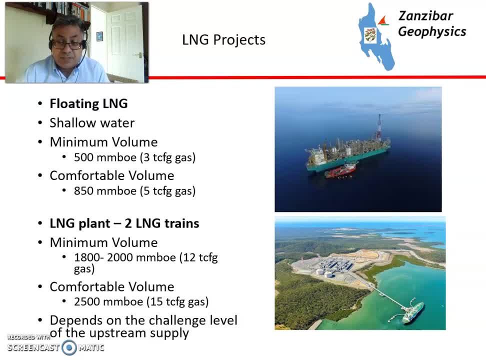 about five tcf of gas. Again also depends on the liquids that you will get with the gas. If you're looking for an abundant volume of liquid gas, you'll need a minimum volume of about 12 tcf of gas. but those are rough figures that you would want. Again, some of these things can be extremely large. 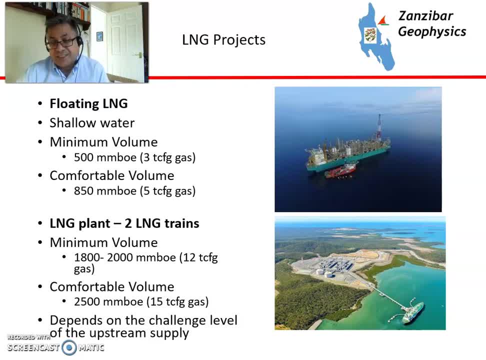 like Prelude, with extreme levels of complexity. For a liquefied natural gas plant onshore you'd want a minimum volume of about 12 tcf of gas, comfortable about 15 tcf of gas. It kind of depends on the challenging level of the upstream. so if you've got a complicated situation in terms of upstream, 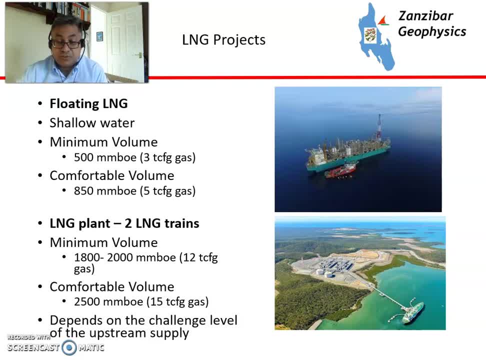 expensive facilities. you'd want a bit more in terms of volume. also, if you're in a situation where it's relatively remote from other areas, there's unlikely to be any third-party business, then you'd obviously want a little bit more volume. but this is a rough figure that you would want to have to make a. 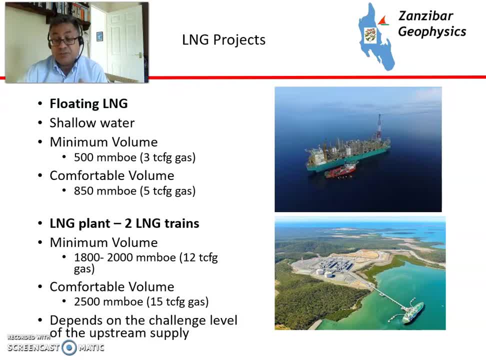 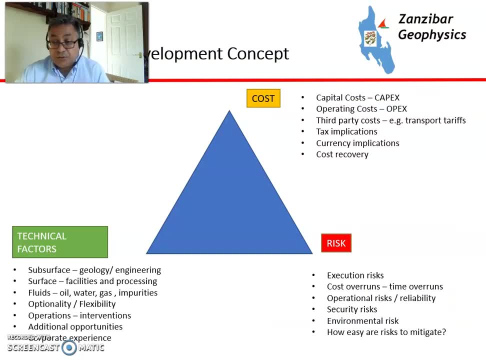 project work. obviously, the more you have, the better it is, because the more margin you have. so, to sum up, when you're selecting the development concept, you got three basic sides of the triangle. you've got your costs: your capital costs, your operating costs, any third-party costs in terms of tariffs, tax. 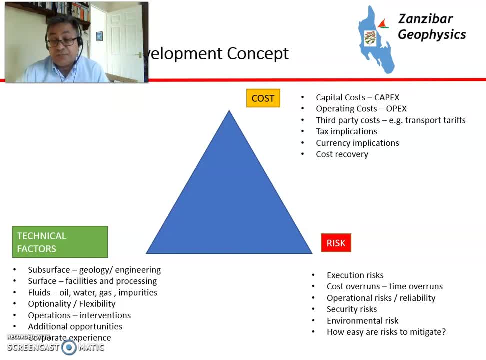 implications, currency implications and cost recovery if you're within a PSA environment and all the fiscal implications go with that. you also have your technical factors: subsurface geology, engineering. obviously, as geologists, that's what we concentrate on. but it's not all that. but that isn't. 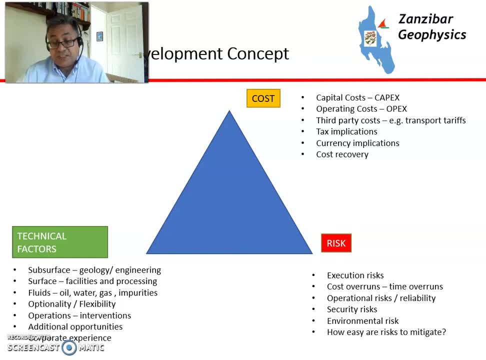 everything you have, your surface facilities, processing what processing you need to do. are there any nasties within the field? so, for instance, my captains, h2s, excess co2, etc. that you will need to process and dispose off in a safe manner? optionality and flexibility are things likely to change, as any third-party business that may come. 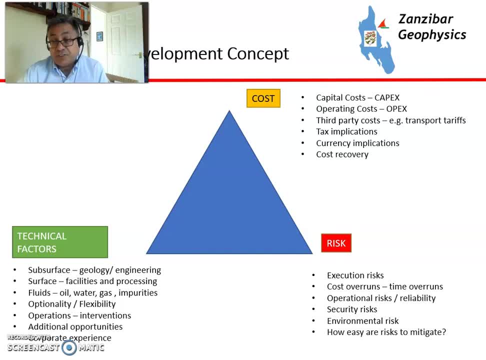 operations and interventions will you be needing to enter your well, for example, if you have a subsea well, they're very difficult to enter, the very difficult to to work over. If you have a well-normally planned platform, a lot easier to work with. 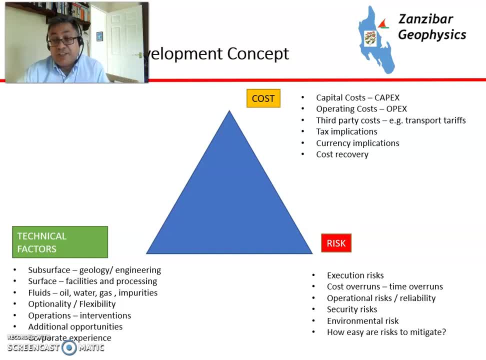 Still hard but easier. And also, are there any additional opportunities, whether they're something that you own yourself in terms of satellites, or is it any third-party business, Any corporate experience? What are you engineers good at And how much novelty can you work? 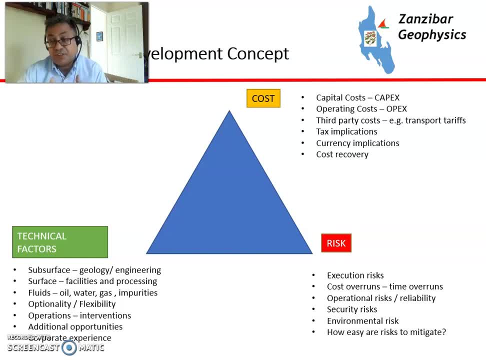 with. Obviously, the more novelty you have, the harder it is to execute effectively, which comes back to the risk in terms of execution risk, How easy is the project to do? If it's something that you do relatively routinely, okay, it will have risk, but it's something. 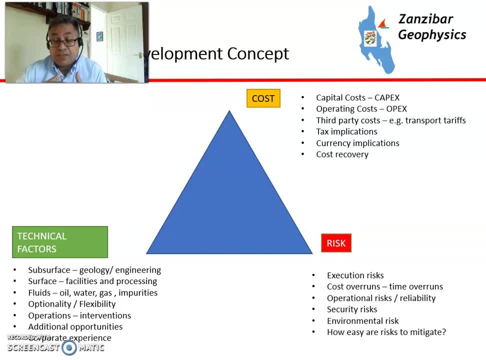 that you can do, that you will do If you have a lot of novelty a bit harder to do. that Cost overruns, time overruns. Projects tend to overrun by cost and time. Very few projects do it successfully and people always overestimate their capabilities, Operational risks in terms 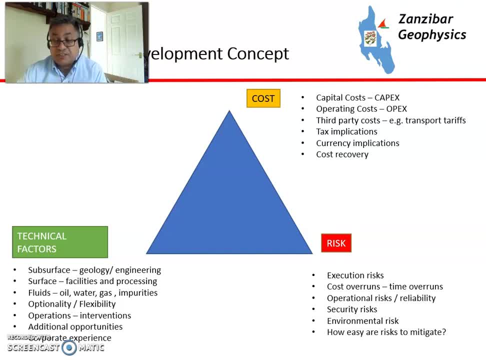 of reliability, Security risks in terms of reliability In terms of where you're operating at, Environmental risks And how easy are all of these risks to mitigate. So these are the factors that go into selecting a development concept which you, as a geologist, need to be aware of Now. there are experts who know a lot about this. 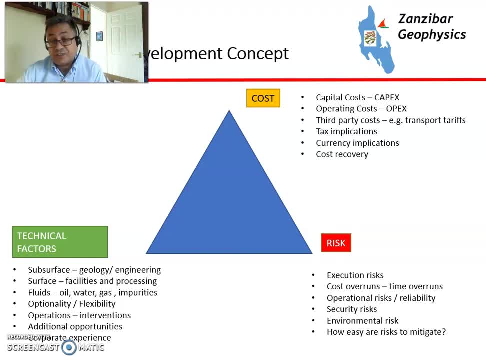 more about this than me. So I really would suggest you contact your friendly neighborhood engineer, your friendly neighborhood economist, and work together to come up with the right solution. Thank you very much.